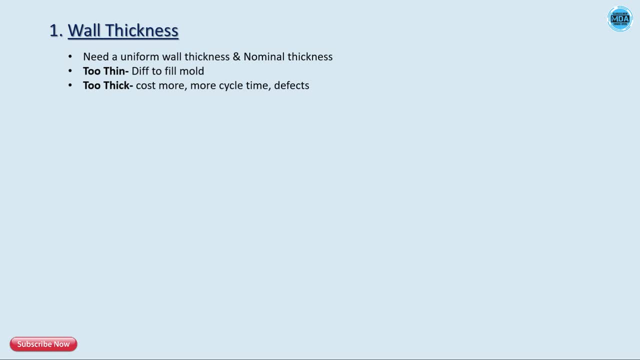 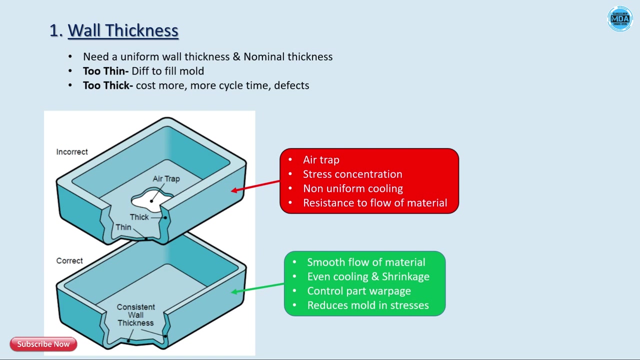 thickness, it will difficulty of filling of material in the cavity of mold and if you consider too thick wall thickness then it will directly impact on the material cost and wastage of material and also defect in the final product. so the quality will be less here and the mold cycle time also increases for too thick. 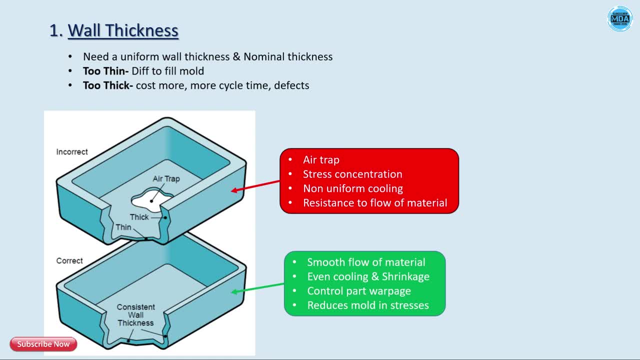 wall section. so the nominal wall thickness here plays very important role in the plastic product design as per the cost, quality and the defect point of view. so what is mean by nominal wall thickness? nominal wall thickness is nothing but the minimum wall thickness that satisfy the functional and the assembly requirement. so 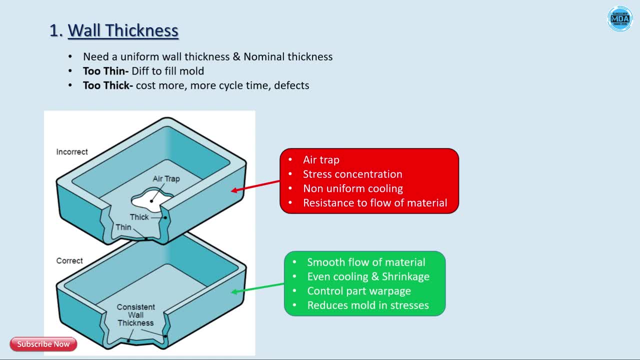 to consider a proper wall thickness. there are, there are certain parameter which depend, which depends on the wall thickness. first one is a strength requirement, assembly requirement, which is nothing but the fastening force we consider here, and the loading and the material and the dimensional stability. so the ideal guideline here is to keep the wall. 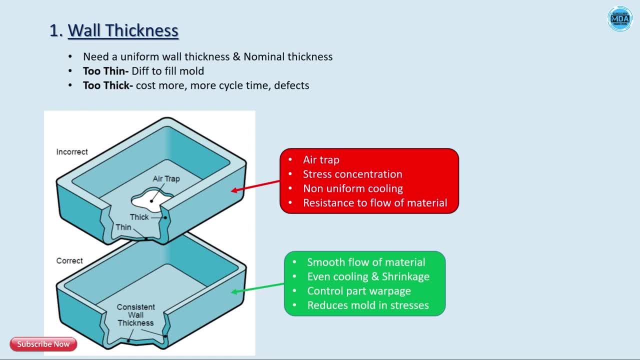 thickness uniform throughout the all section and generally the nominal wall thickness for the plastic part is 2 mm to 5 mm, but commonly we we use 3 mm to 5 mm in the range, as per your requirement. you can consider the wall thickness of rib and the ball. 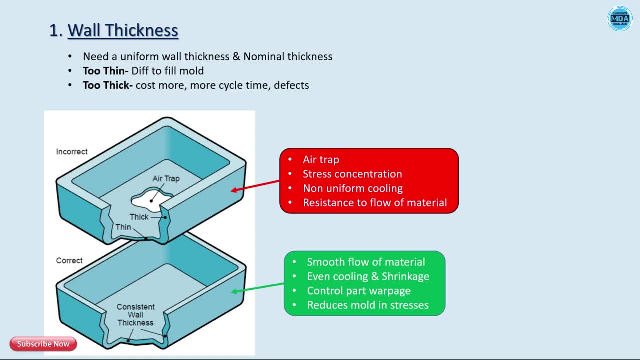 thickness or you can go back and check the barrier at the wall thickness. you can also consider we're using 3 mm to 5 mm thickness, so that should help. this is Mant mass of the wall thickness and we can do any kind of mesh and not lose this thickness. so the recurring воp use so that isом. 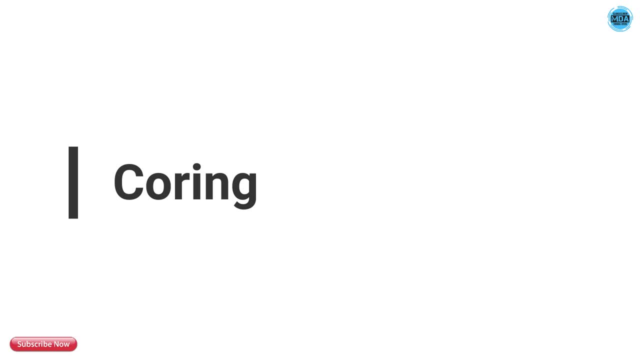 for this product, the minimum lower the wall thickness. the remaining wall should not be too thicker because it will affect on the appearance. surfaces like used to maintain the uniform wall thickness. so what is mean by coring? coring is nothing but the removing of unwanted material from the part for your 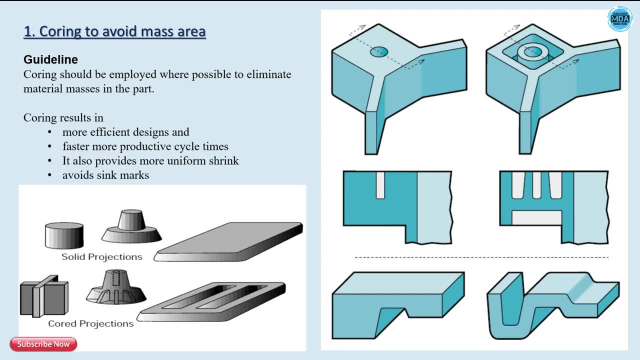 good, good understanding. you can see this picture how we modified the part and remove the unwanted material. so coring help you in a material reduction and also it will reduce the defects number of defect that will cause due to thicker section, like a shrink mark is there. it will reduce the cycle time and 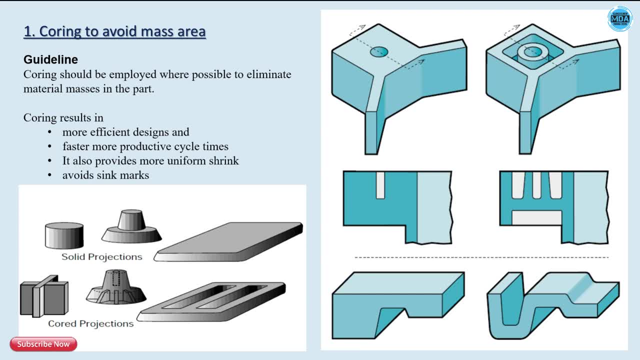 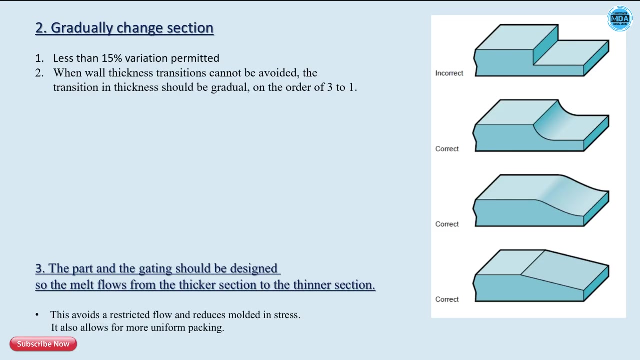 if you consider the uniform wall thickness, then there is an uniform cooling. if you consider a coring and maintain the uniform wall thickness with the help of coring, that design is is- we can call it as a effect value design. as per the process, during design we must avoid all the corners and sudden 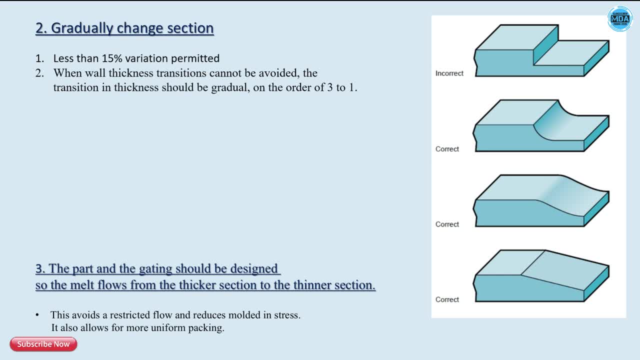 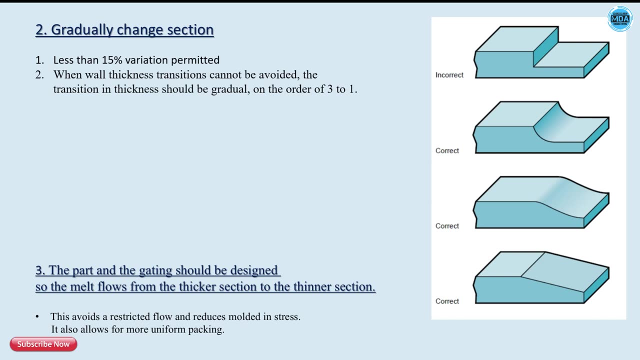 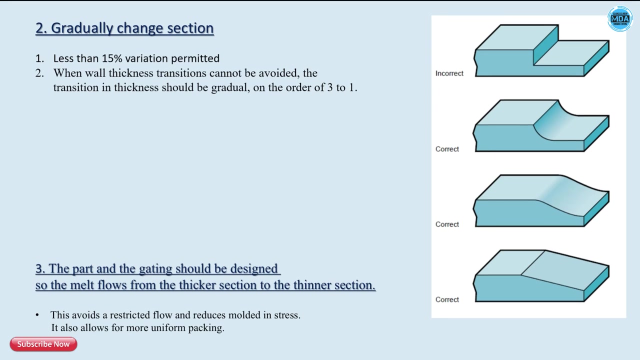 drop section. because of this there is a stresses in the mold and there is there is no proper flow of material. so simply by adding the radius or gradual change in the design, we can avoid this defect. so the recommended thickness variation is less than 50 percent is permitted. so the less than 50 percent variation in 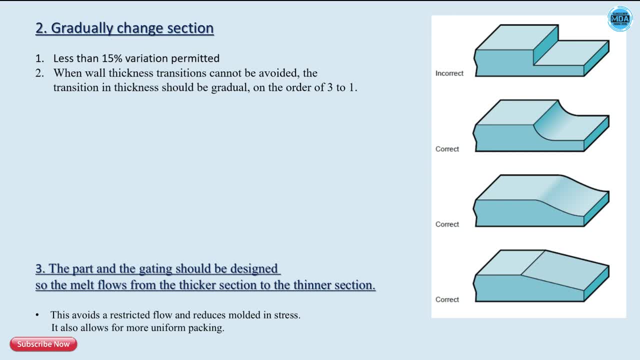 the thickness of two section is permitted here. and about the gate location. the gate must be located in a such a way that the flow of material from a thicker section to the thinner section, so that it allows more uniform packaging or filling of mold. parting line: parting line is a nothing but the 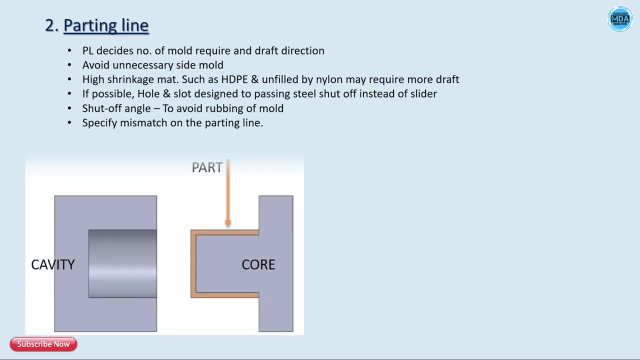 common line between two or more mood like core, cavity slider and the lifter. so what is mean by core and cavity slider? lifter in the mold, as here in the picture, you can see that core is a excluded part of the mold and cavity is nothing but the depression in. 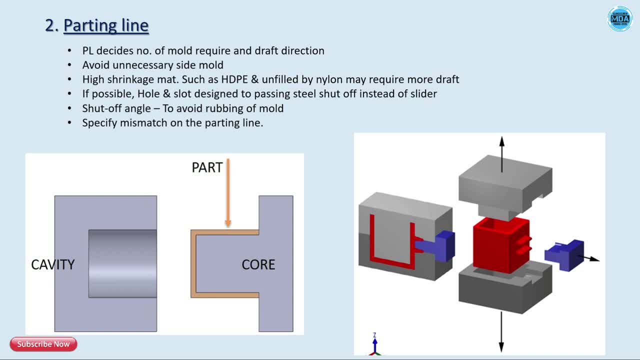 the mold slider are required to remove the side feature. suppose we are unable to eject the feature from core and cavity, for that we use the side core to remove that feature from the side lifter. so lifter is same like a slider but lifter with the mold lift lifted and take out. 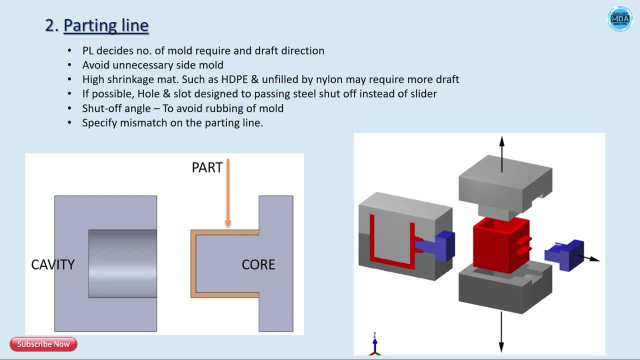 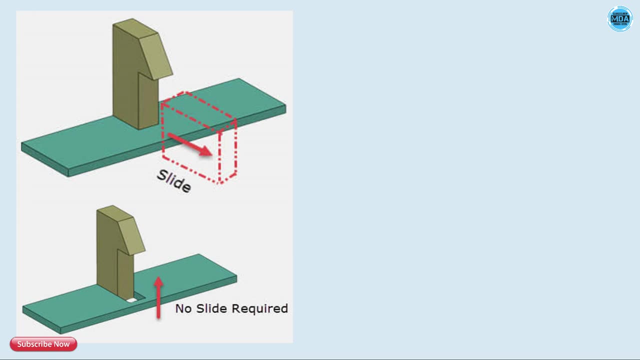 the undercut feature. so with the mold lifter is lifted and after that it will remove from the mold mold. so it will. it will take the undercut part. here in the snap fit example you can see that by simply adding cutout or by coring at the bottom. 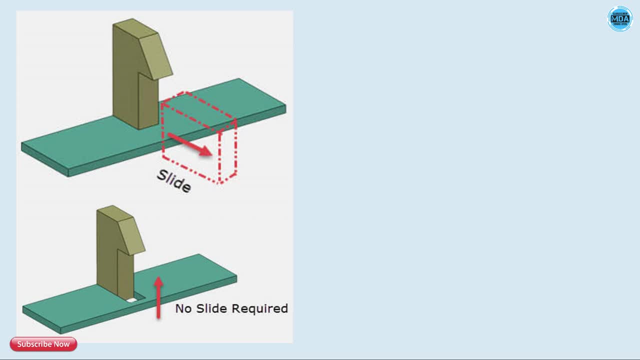 we can avoid the slider if you cut out like this. we can avoid the slider but first check the functionality of feature and then take the proper action that will not affect the functional requirement. so we need to consider the functional requirement before cutout or changing the parting parting line also. 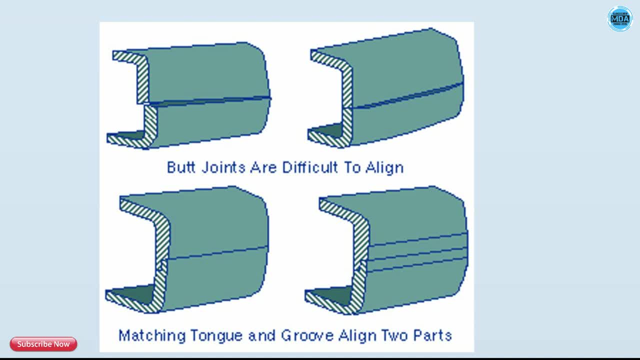 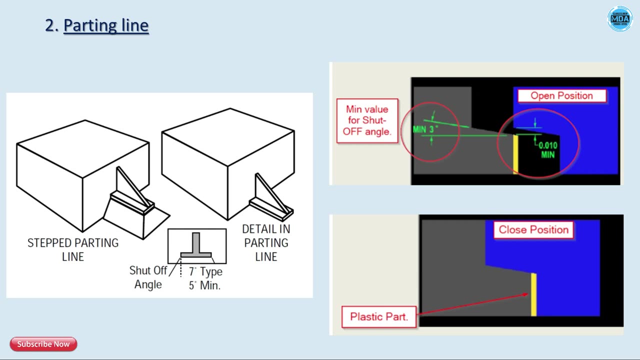 for a proper mating or for the proper assembly of mold. we can add mismatch feature in the part like Tunk and grow or the step. also, there is one more term related to parting line is shut off. so what is mean by shut off during assembly or during ejection of mold? 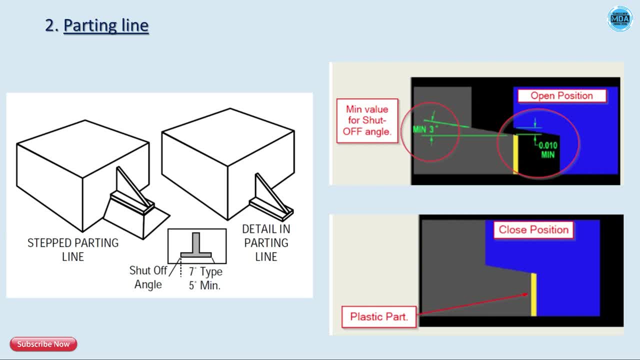 there is wearing and tearing of mold, which, which decreases the life of the mold, is called as shut off. we can avoid the wearing and tearing of the mold by simply adding or applying the draft to the shut off surfaces and we can call that shut off surface. angle is: 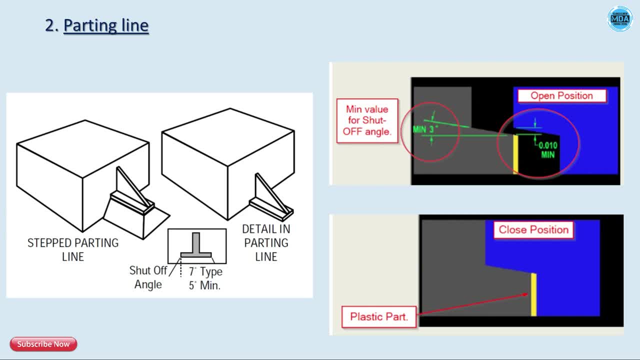 called as shut off angle and the angle with the avoiding wearing of tearing of the mold is called as shut off angle, as in the picture. you can see there the actual meeting, the core and cavity in contact to that surface of the part, that surface of the mold we can give the shutoff angle. there is a complete 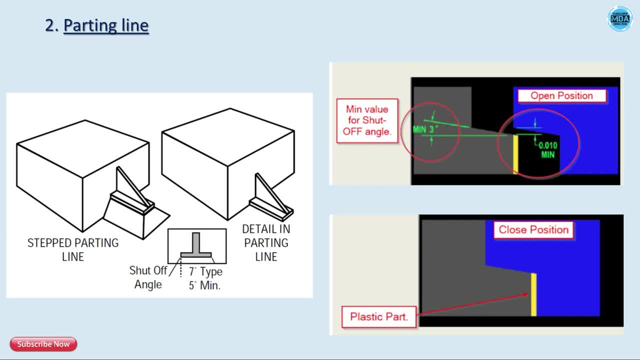 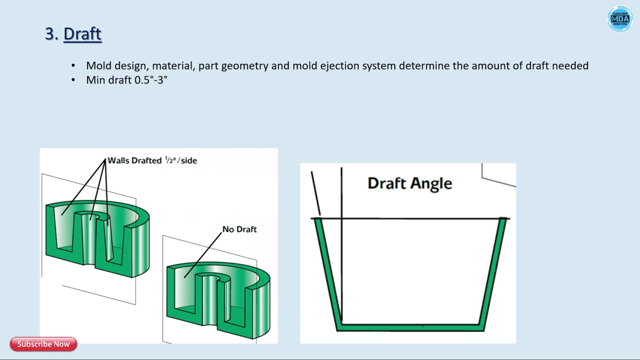 contact between the mold and the, that is, core and the cavity. so the recommend shutoff angle is 3 to 7 degree and we generally, commonly we we use the shutoff angle is 3 to 5 degree. draft. we apply draft angle to all vertical surfaces which are 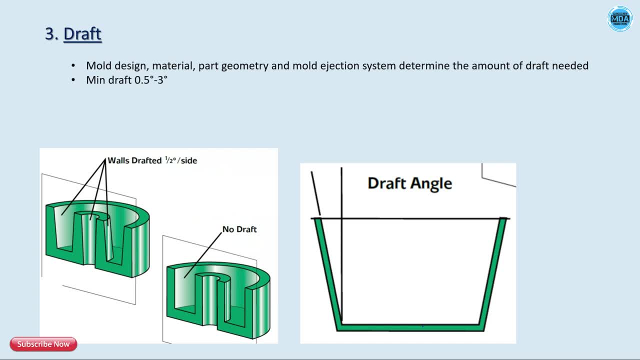 perpendicular to the parting line or in the direction of pulling to easily remove part from the mold. it is generally good practice of applying the minimum draft instead of no draft. so we need to apply draft to all surfaces and perform draft analysis before deliver the part to the mold designer. so the 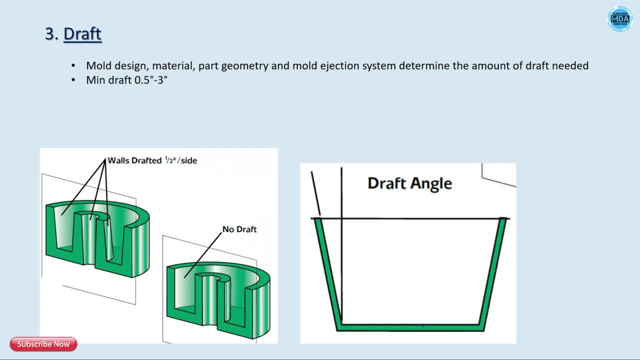 recommended draft angle is 0.5 degree to 3 degrees recommended but it depends upon the height of the surfaces. we need to check that. how much material is adding on the bottom side or how much material is a remain on the top side. so depending on that we apply the draft undercuts. what is mean by? 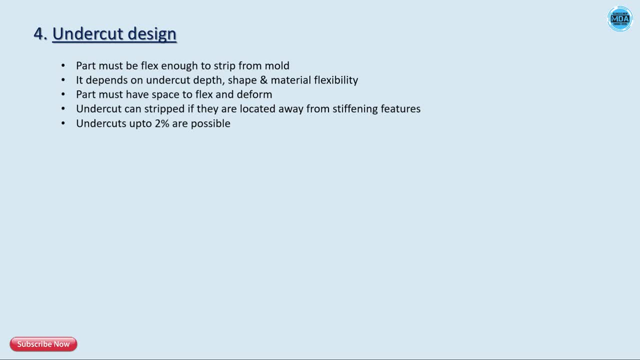 undercuts. I think you will know already, but shortly we will revise the definition. so undercut is nothing but the those feature are unable to eject from the mold. the feature is called as undercut. for undercut the feature alignment is not perpendicular to the mold parting line, so the undercut feature is not in. 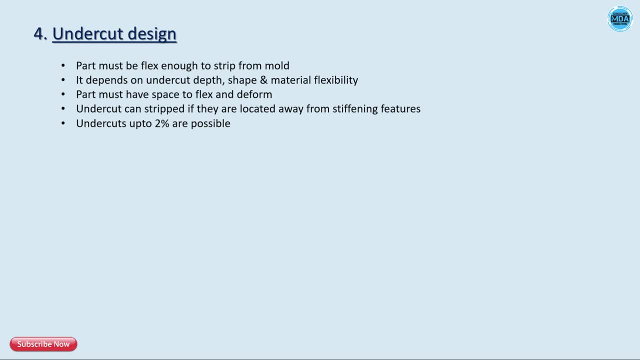 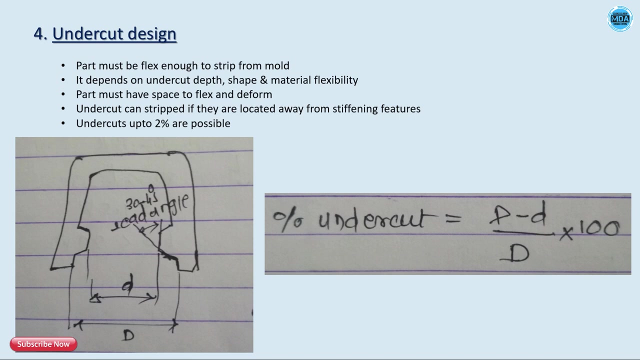 the alignment of parting line. not perpendicular to the parting line, or you can see that- not in the direction of pulling direction. firstly, our aim is to avoid the undercuts in the part, and sometime we can eject the undercut from the mold also. for that the material must be flexible enough and it depends upon. 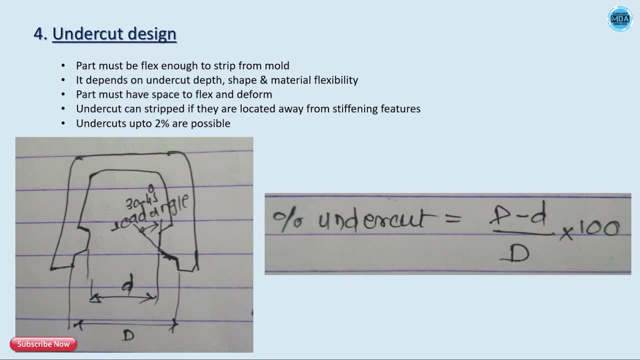 the shape of that part and its material. material of the part and the undercut feature must be away from the stiffening area, that is, from the bottom side of the part, from the ribbing area or the corner areas, and we can calculate the percentage of undercut by using this formula, as you can see here, and the 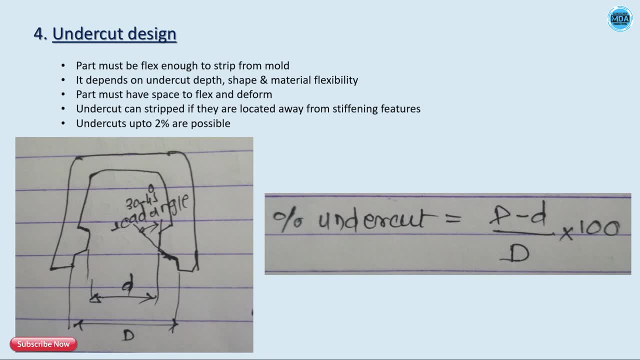 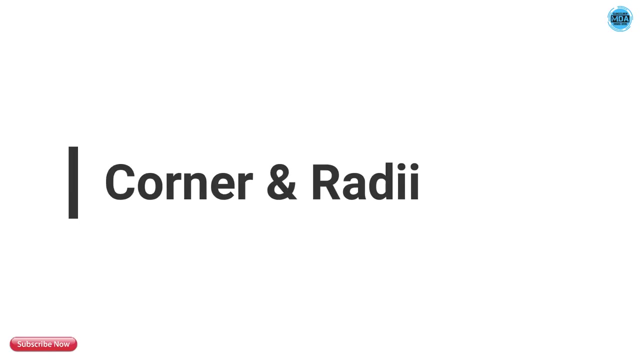 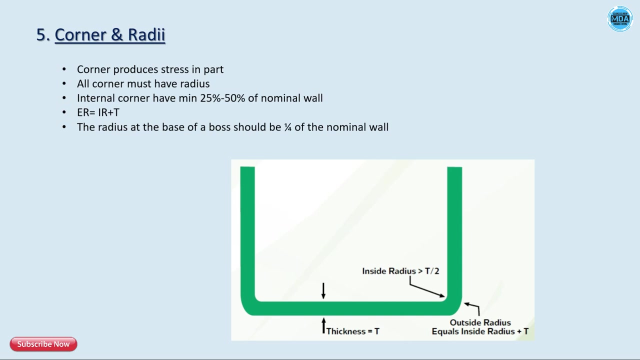 undercut. up to 2% are possible in the part and it varies with the material to material. generally, the generally we avoid the stripping of undercut for stiff like polycarbonate. polycarbonate paint and the polyamide corner and radar corner produces the stresses in the part. so by simply adding the radius we can avoid the stresses due to radius. 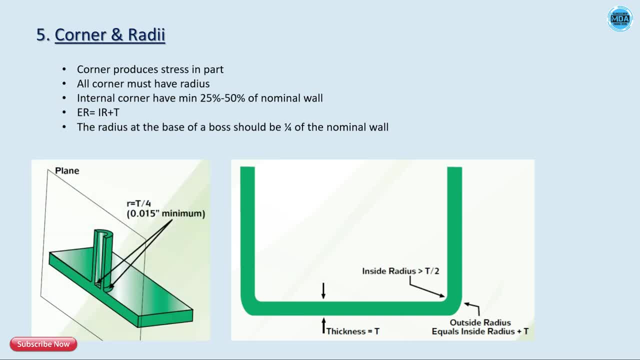 there is a smooth flow, smooth flow of material in the mold and by adding the radius, keep in mind we need a uniform thickness, so for that we can refer: external thickness is equal to internal thickness plus radius. to maintain the uniform thickness generally, the inside radius should be greater than 50% of wall thickness and the radius at the bottom of 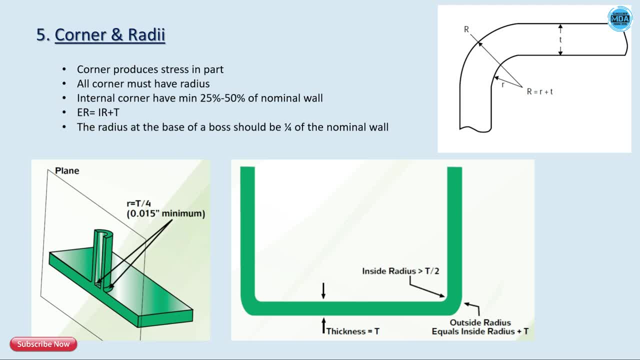 the boss is equal to 20% of the wall thickness, and, and, And. the minimum radius at the bottom we can keep is 0.3 to 0.55 times of T, That is, 30 to 50% of wall thickness. Boss design. 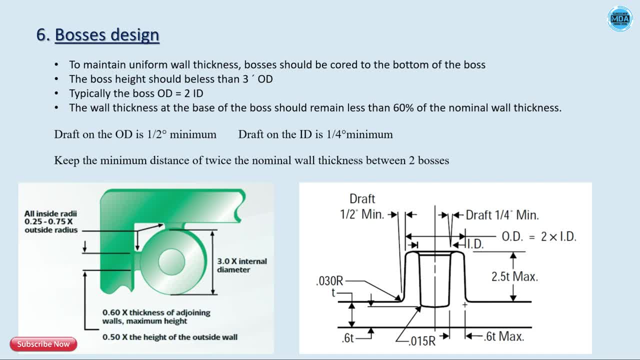 Boss is a mounting feature in the plastic part. So the design requirements for the boss are the minimum radius at the bottom, 0.3 to 0.5% of wall thickness, That is, 30% to 50% of the wall thickness. 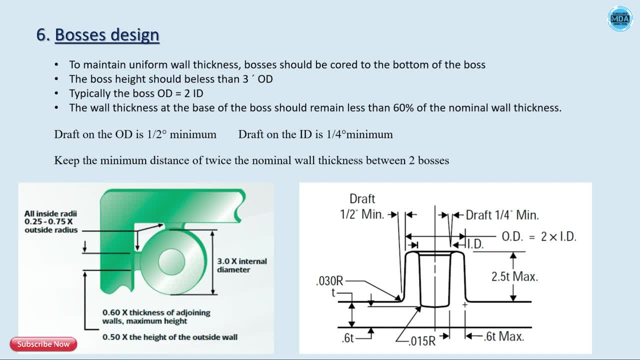 And the spacing between the bosses is 2 times of the wall thickness. Radius at the base of the hole is 25% to the 50% of the wall thickness. Minimum draft on the outer diameter is 0.5 degree And the minimum draft on the internal diameter is 0.25 degree. 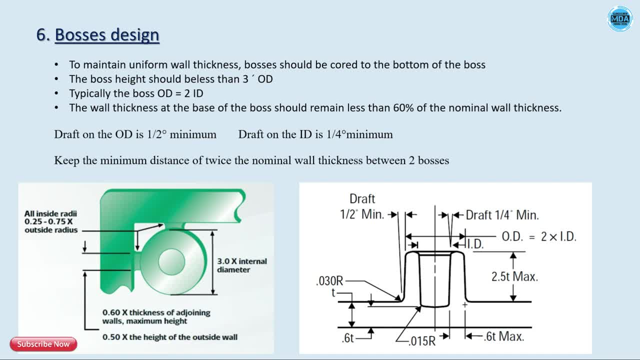 Radius at the tip of the boss is minimum value. to reduce the stresses, You can choose the minimum value, that is, 0.1, 0.2,, 0.5, 0.3.. Jumper at the top of the boss. 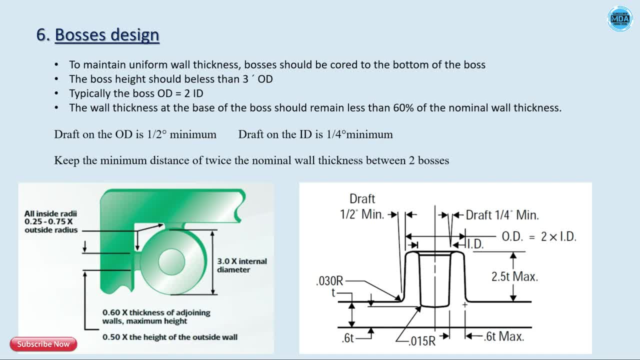 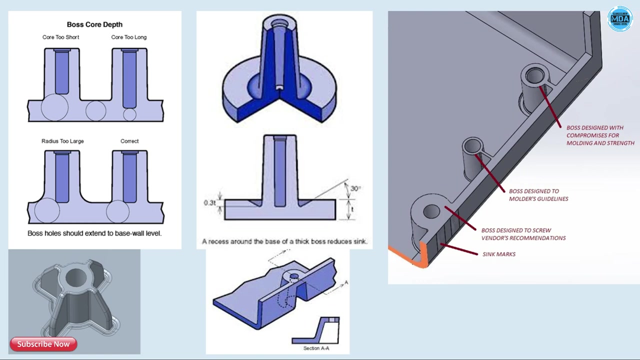 For the good lead. for the fastener. Entry point for the fastener. you can see The wall thickness of the boss should be less than 60% of the wall thickness. Or if we are adding the boss on the surface A, then at that time it is less than 50% of the wall thickness. to minimize the shrinkage. 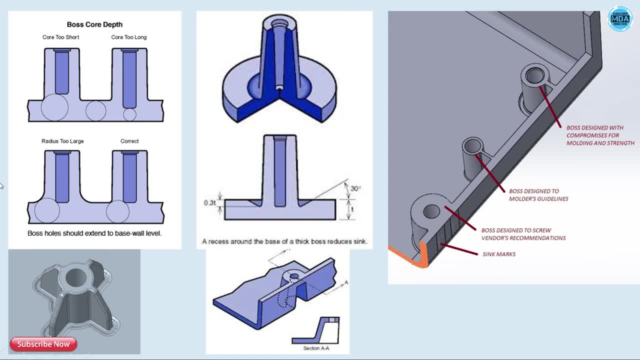 If The wall thickness of the boss is greater than the nominal wall thickness then it will create the voids sink mark and it increases the cycle time. Boss creating the mass area need to be core out and attach boss to nearest side wall or create the side rib or gusset around this to provide the stiffness to the boss. 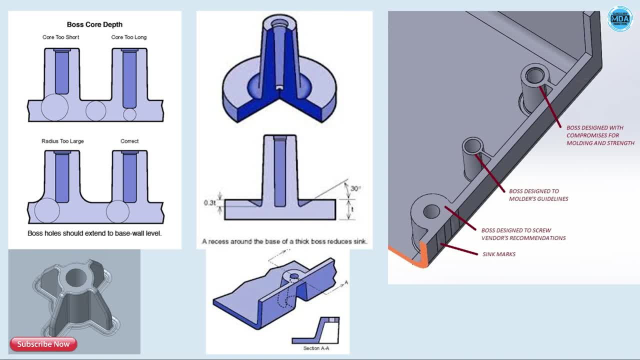 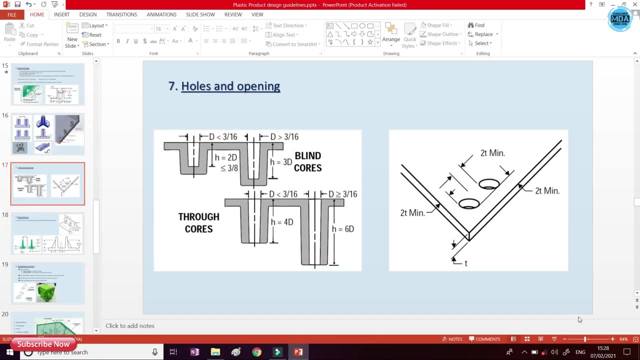 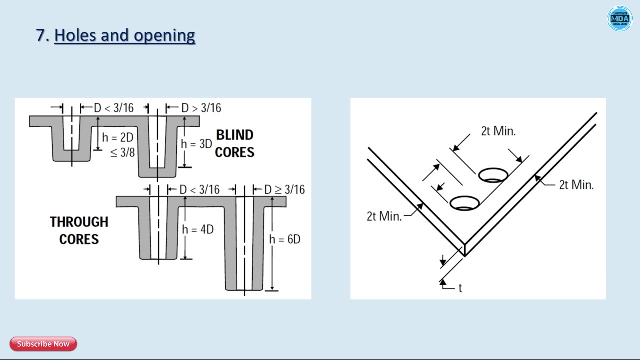 Here we need to avoid the mass area and maintain the uniform thicknesses or in the proper variation. There are two type of holes. One is a thru hole and the second is a blind hole. Generally We use core pins in the mould to create the hole in the part. 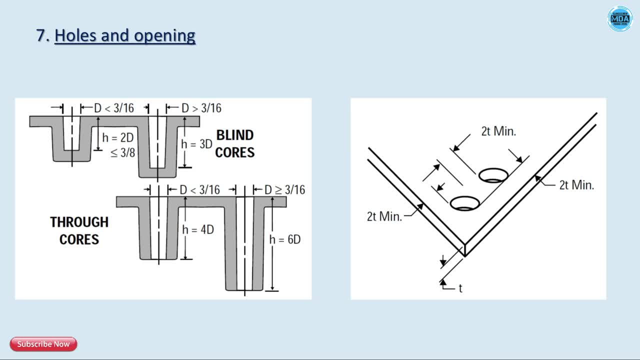 Generally we use core pins in the mould to create the hole in the part. So Then Core pin for a blind hole supported from one end only, And for a through hole we need to apply draft and we can eject from core and cavity. So for through hole, we can eject from core and cavity only. 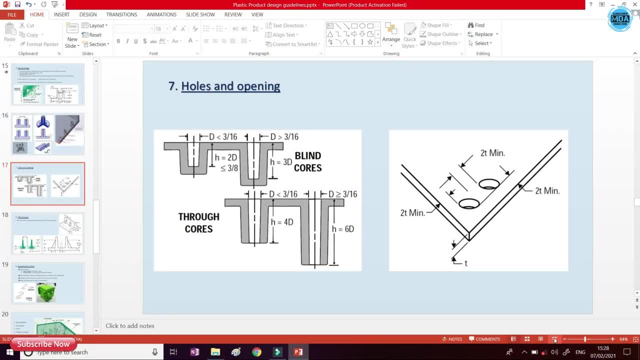 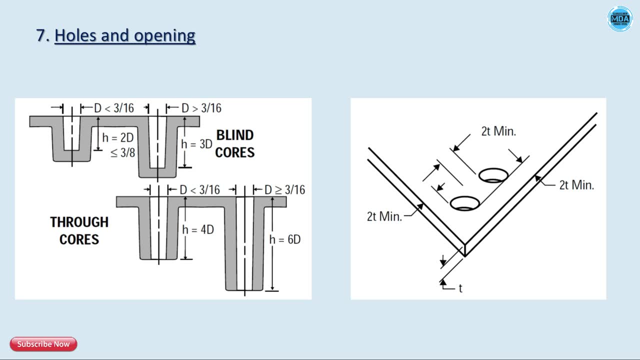 And for a diameter less than 3 by 16 inch, the depth of blind hole is equal to 2 times of diameter of the hole, And for a diameter greater than 3 by 16 inch, then the depth of blind hole is 4 times of diameter. 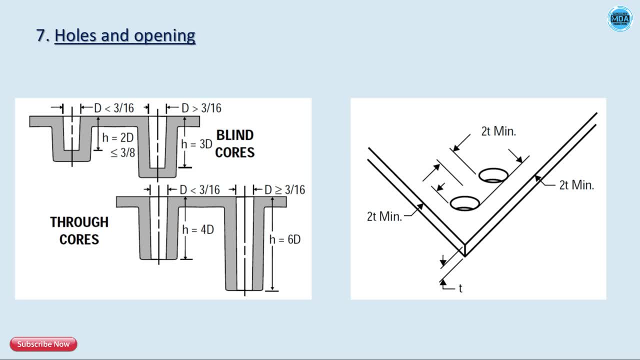 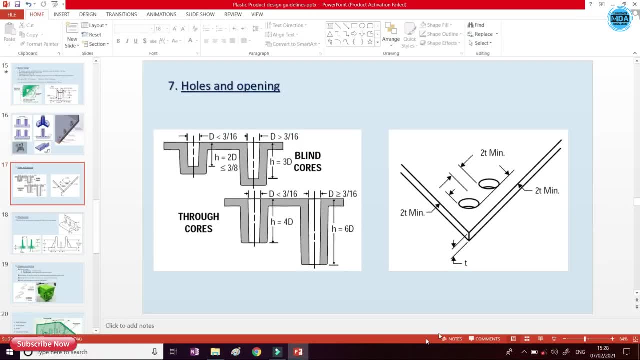 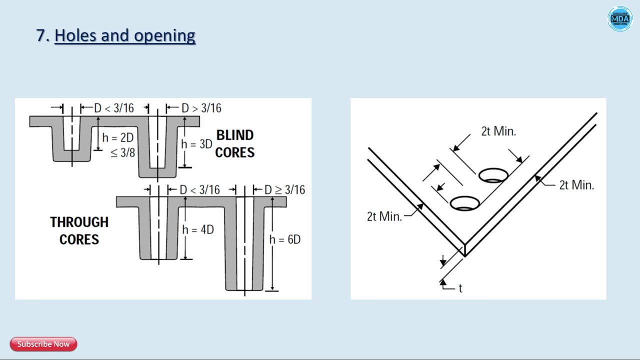 And the distance between two hole from edge to edge should be at least 3 by 16 inch, 2 times of wall thickness, And always try to eject, hole or slot in a core or cavity instead of slide action, which required cam or pull core action that will increases the cost. 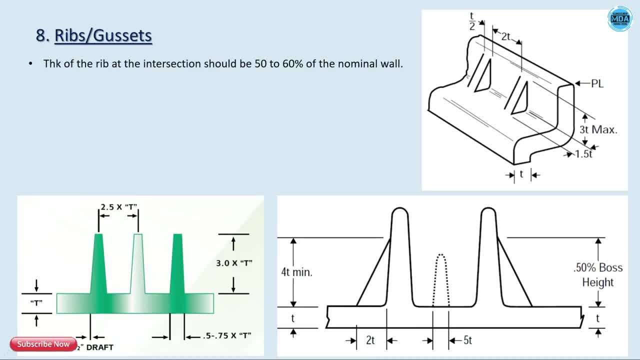 Ribs, As we know that the ribs are used to provide the strength and stiffness to the part. So if you want the stiffness, Then you can add the rib to the particular area to stiffen the part without increasing the wall thickness. So 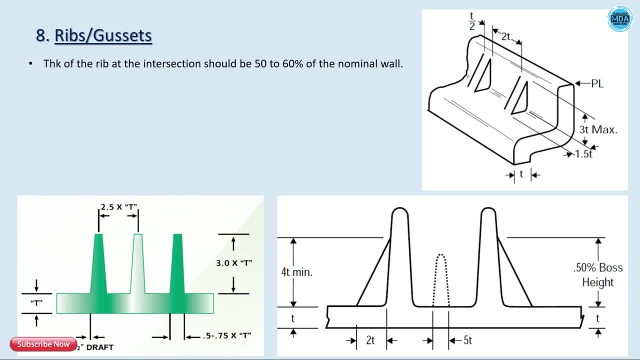 Here you can see that The thickness of the rib should be less than the nominal thickness. For high shrink material it will be less than 50 percent of wall thickness And for a low shrink material it will be less than 75 percent of the wall thickness. And the height of the rib should be. 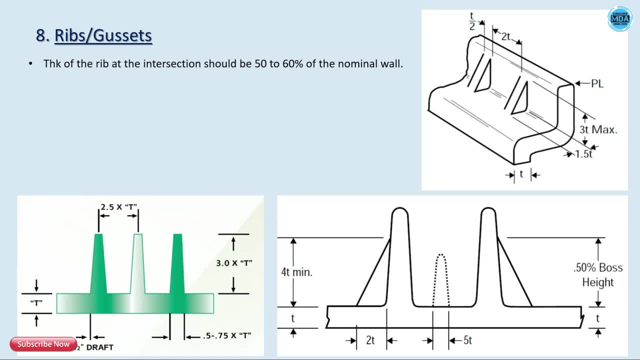 2.5 times of wall thickness And the distance between the two ribs should be 3 times of the wall thickness. And try to use multiple small ribs instead of one large rib. To stiffen the boss, We can add the rib along the boss.